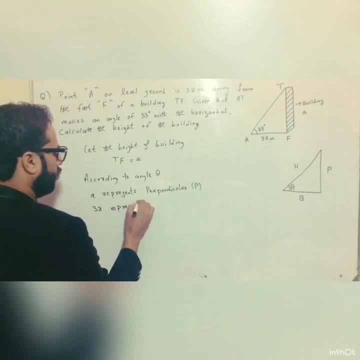 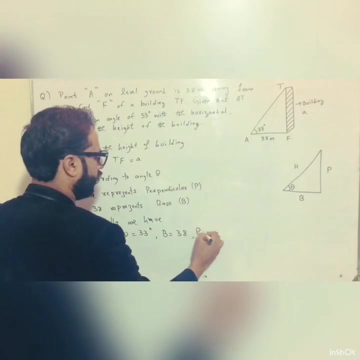 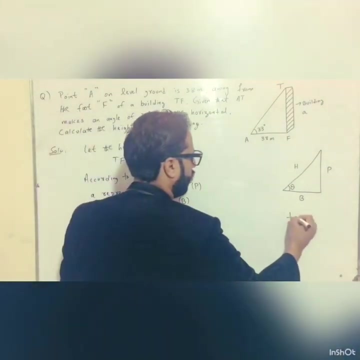 38 represents base, which we can write it as B. So finally we have: theta equals to 33 degrees, base equals to 38 and perpendicular equals to A. Now the suitable combination to find this. We have: tan of theta equals to perpendicular over base. 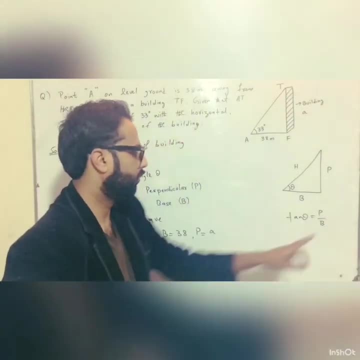 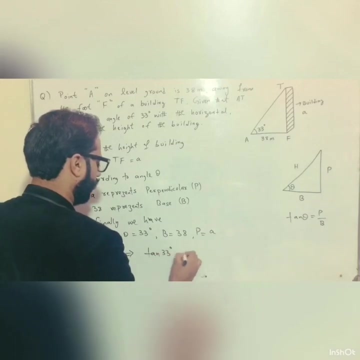 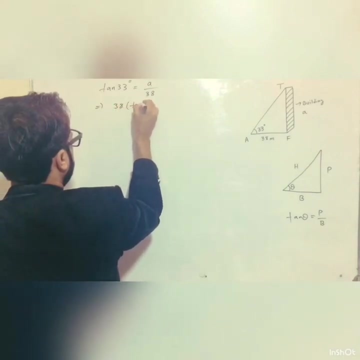 So we have theta, we have perpendicular, we have base. So apply this formula: Tan of 33 degree equals to A over 38.. Apply this: 38 times tan of 33 degree equals to A. So 38 times tan of 33 degree equals to A. 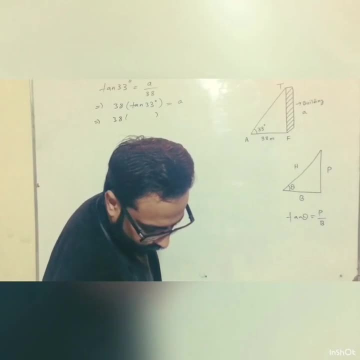 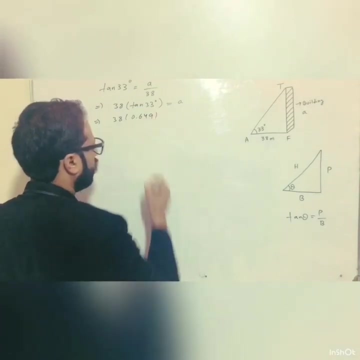 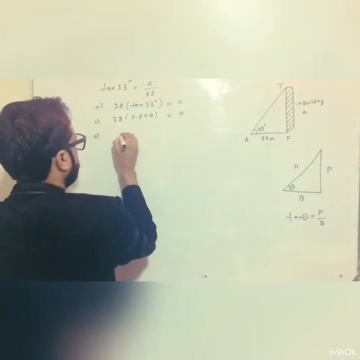 So 38 times tan of 33 degree equals to A. So 38 times tan of 33 becomes 0.649.. You can find this value with the help of a calculator. So this will become finally 24.7 equals to A. 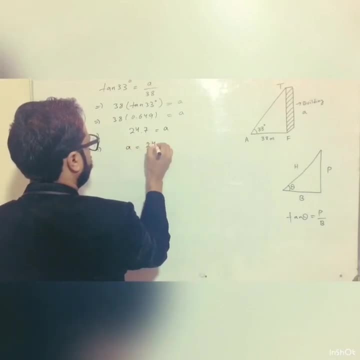 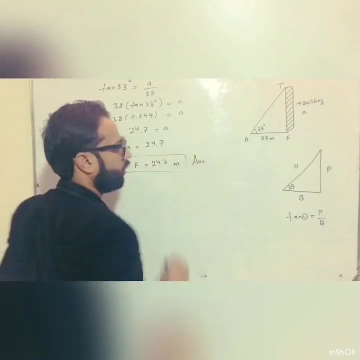 So A equals to 24.7 and A represents the height of the building TF. So therefore TF equals to 24.7 meter. This is your required answer. Another question At a certain time of the day, the church spire PQ. 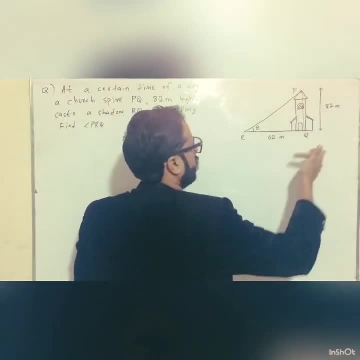 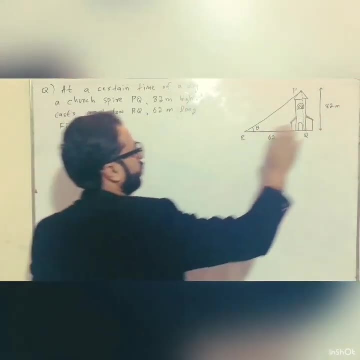 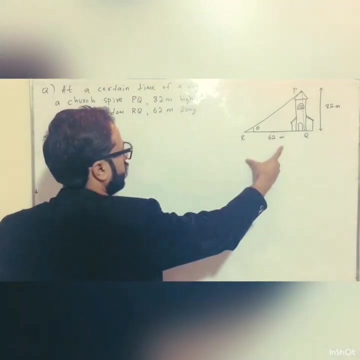 So this is PQ, is the church spire, 82 meters height, The height is 82 meters Cost and a shadow of RQ. If this is PQ, then its shadow will be RQ, So RQ, And it is 62 meters long. 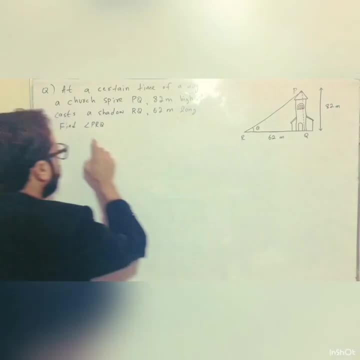 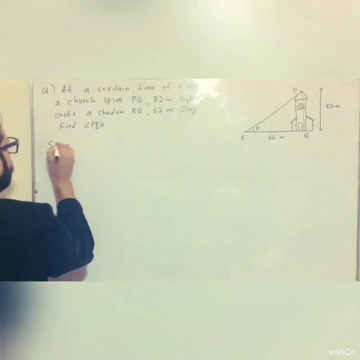 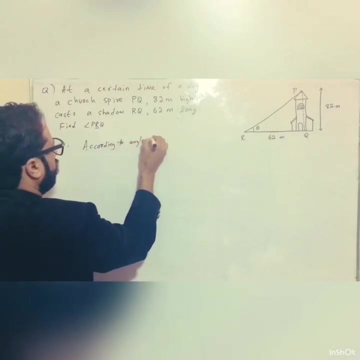 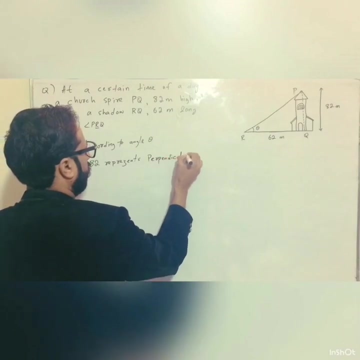 So find this angle. PRQ means we have to find this angle R, This angle R. So let's start the solution According to angle theta. According to this angle, theta 82 represents- Represents Perpendicular, As we are familiar with this diagram. 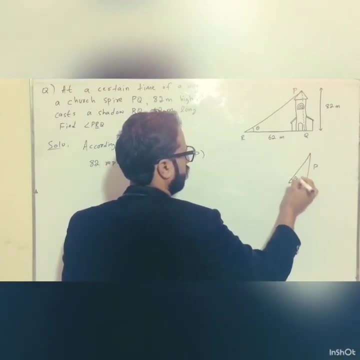 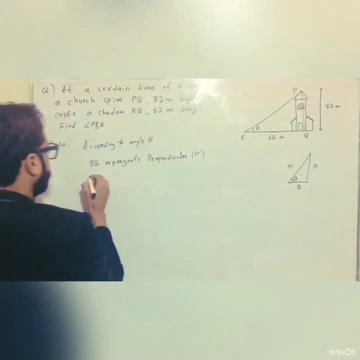 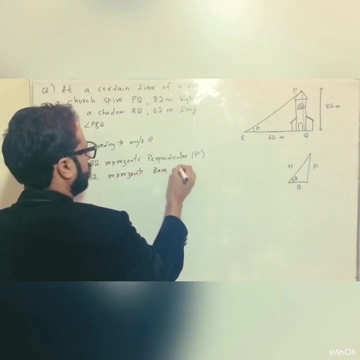 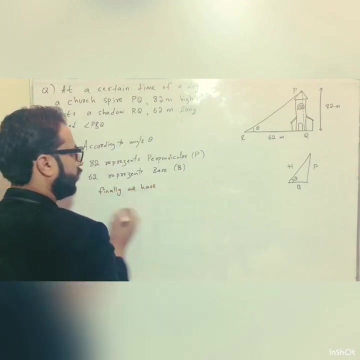 This is an angle theta. It will be perpendicular. This is base And this is height. And, according to this angle, theta 62 represents Base, Which is V. So finally, we have, We have Theta Which we have. 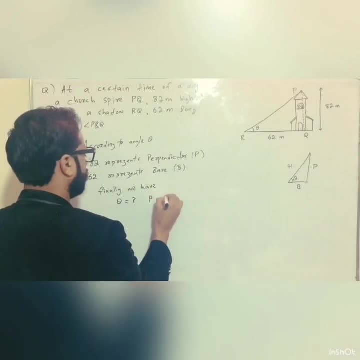 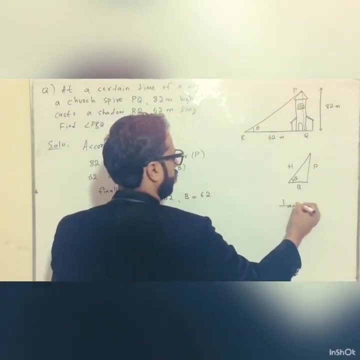 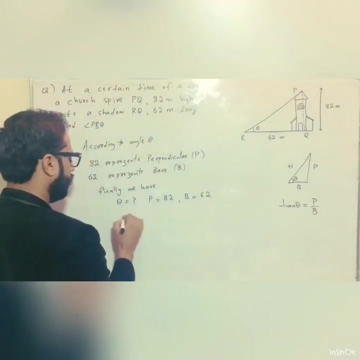 Find: Perpendicular equals to 82.. And base equals to 62.. Again, The suitable option will be: tan of theta equals to perpendicular over base, Because we have a theta, perpendicular and base. So, putting the values, Tan of theta equals to 82.. 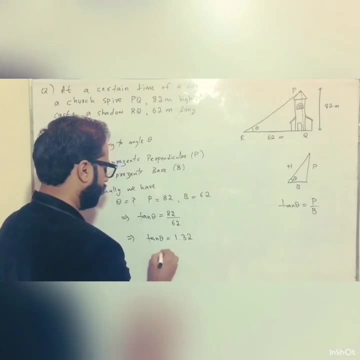 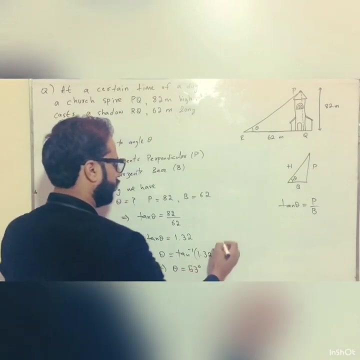 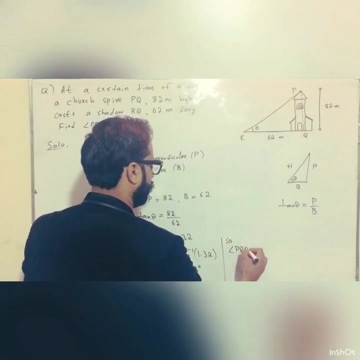 This will becomes 1.32.. Theta will becomes tan inverse of 1.32.. And finally theta becomes- This will becomes Approximately 53 degrees. So Finally we have Angle PRQ Equals to 53 degrees. 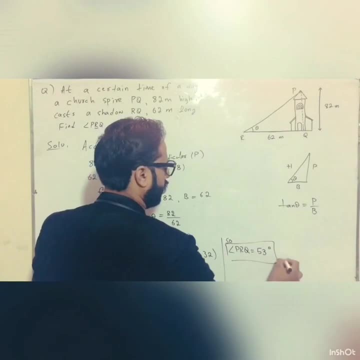 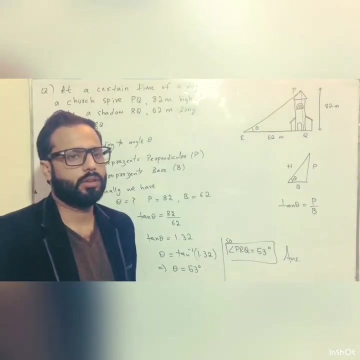 And this is our. So we can see that By using trigonometric ratios We can Solve the Problems Relating to trigonometry in our daily life. So that's enough for today. . . . . . . . . . . . .